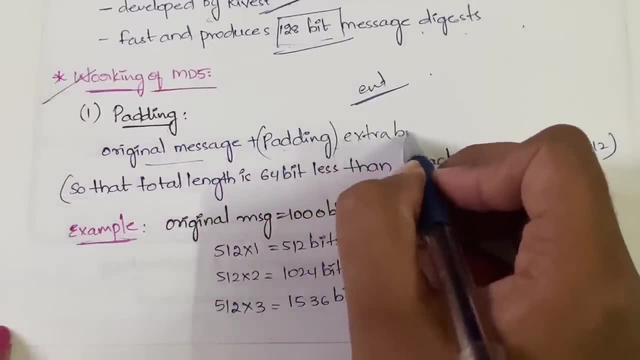 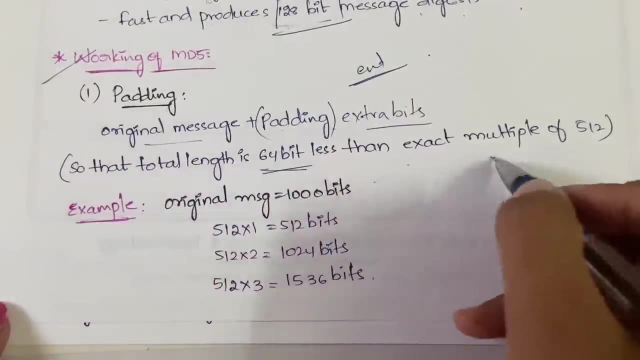 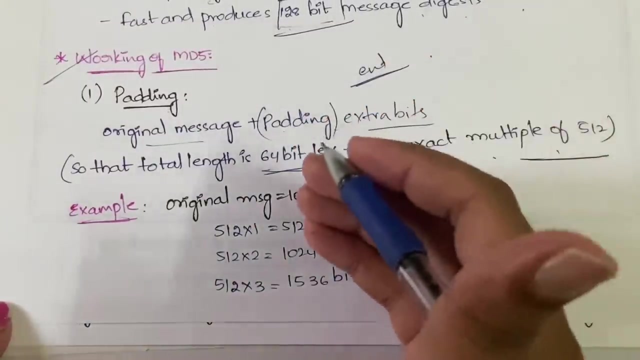 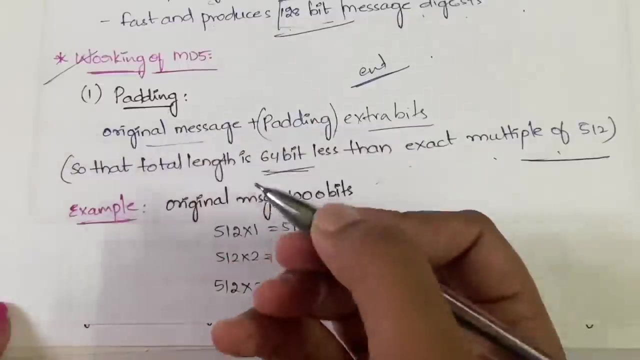 Original message. plus, you will be adding some extra bits at the end. So that is, that is what padding means. Okay, so that the total length will become 64 bit less than exact multiple of 512. Okay, so when you add the number of bits- suppose you add 10 bits, or 20 bits, or 30 bits, whatever it is- when you are adding some extra bits at the end, the total length has to become 64 bit less than the exact multiple of 512.. Don't get confused, I'll tell you. 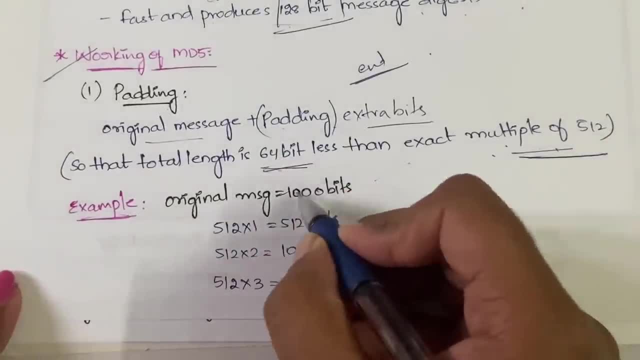 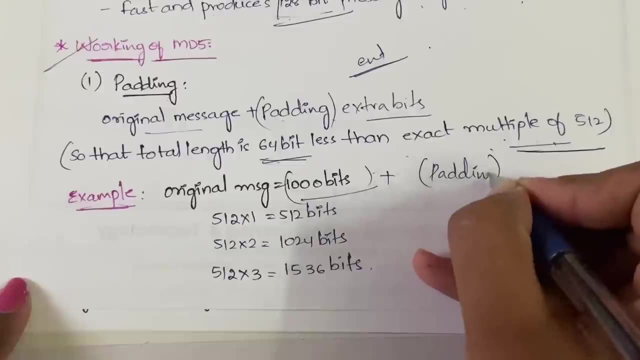 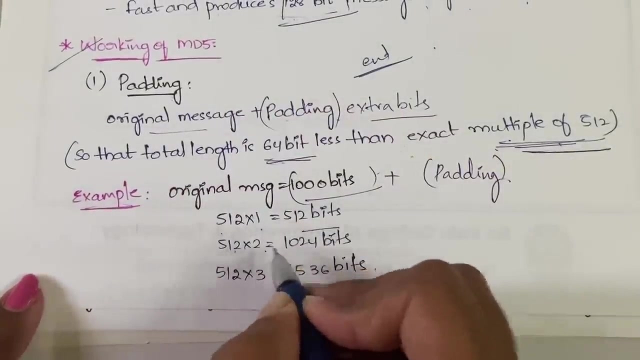 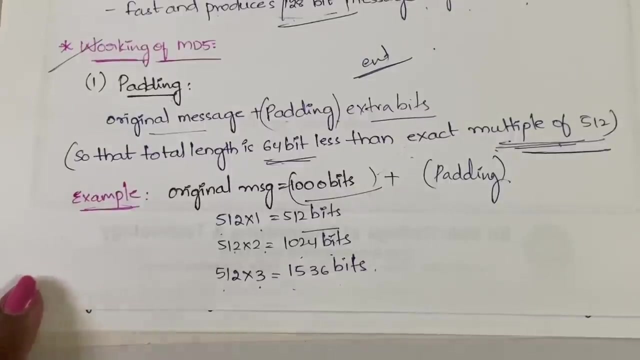 Suppose, for example, let us take we have an original message, then the size of our original message is 1000 bits. Okay, now, plus how many padding bits you have to add, let us calculate, Okay, so multiples of 512, right, So what is? what are the multiples of 512?? 512 times one is 512, 5122 is 1024, 5122, 512 times three is 1536, and so on. you have to do okay, So 512 minus 64. if you do 64 less, he said, right, So 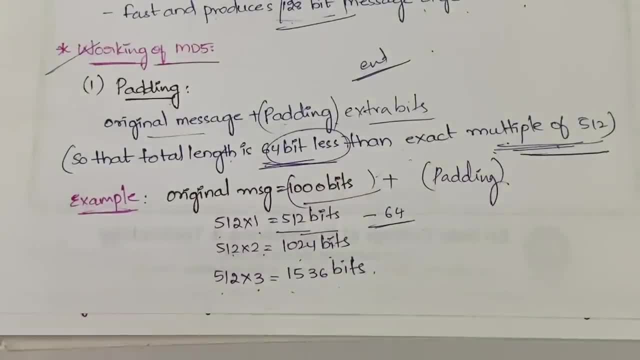 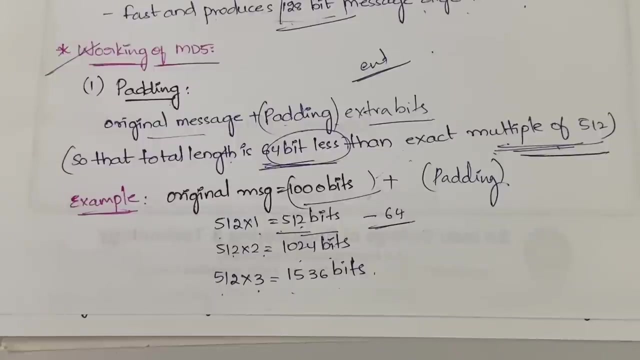 you have to do 512 minus 64. But actually, how many bits you have to total, how what should be your total length? it has to be 64 less than multiple of 512.. So now, if you 512 minus 64, you, if you do it, will become less than 1000, right. So our concept is not less than 1000, we have to get more than 1000, because 1000 we already have, 5000, we have to additionally add some. So obviously 512 times one is 512. 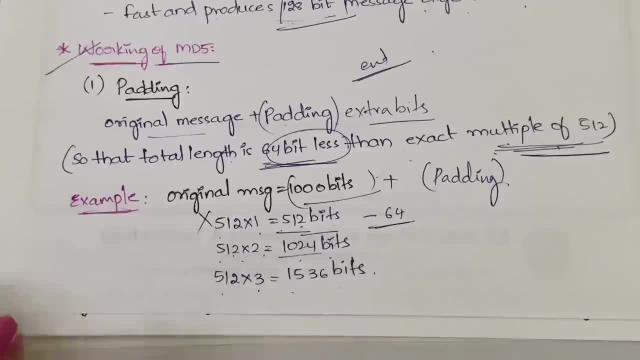 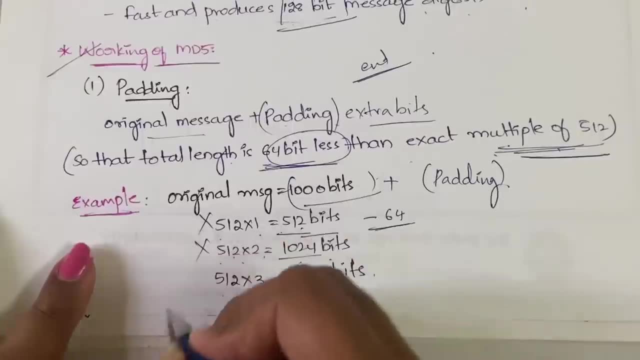 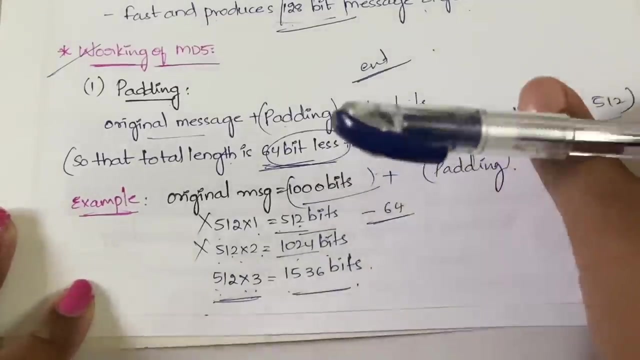 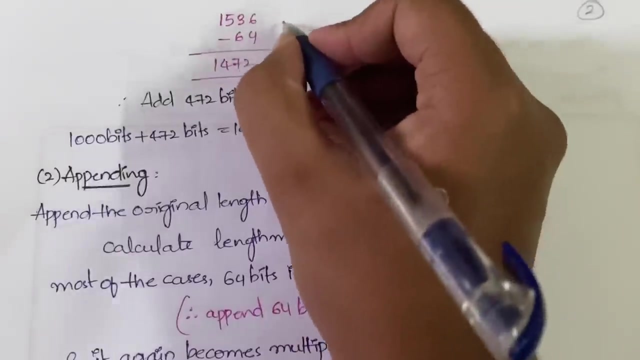 one will not be valid. now, 512 times two is 1024. of course, it is greater than 1000.. But when you subtract 64 from that, it becomes less than 1000, right? so this is also not valid Now. 512 times three. so what is 512 times three? we got 1536. okay, now what you have to do is 1536 minus 64. you have to do: see, 1536 is nothing, but it is 512 times three. okay, now 512. 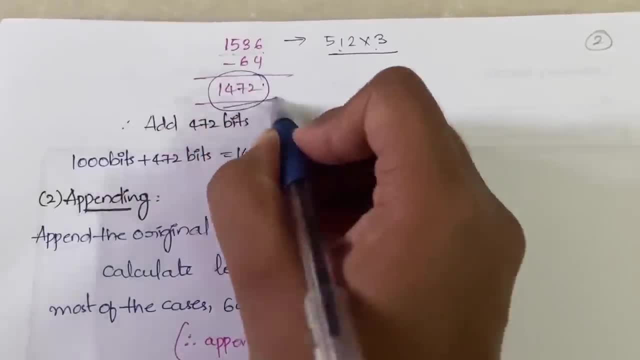 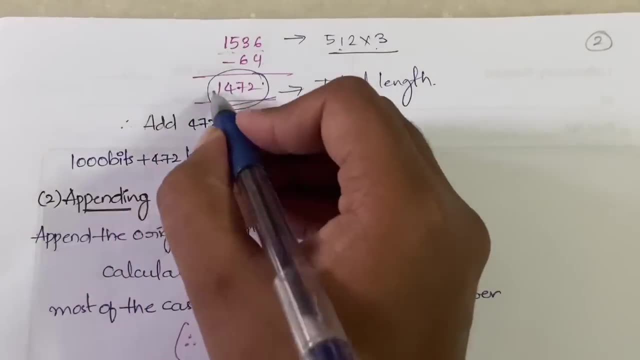 this: 1536 minus 64. you have to do. you will get 1472. what is this? this is not the number of bits that you have to add. this is the total length. got it so: 1472 is the total length, and what is the? 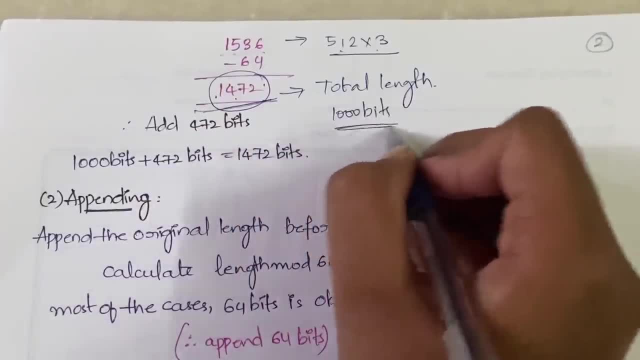 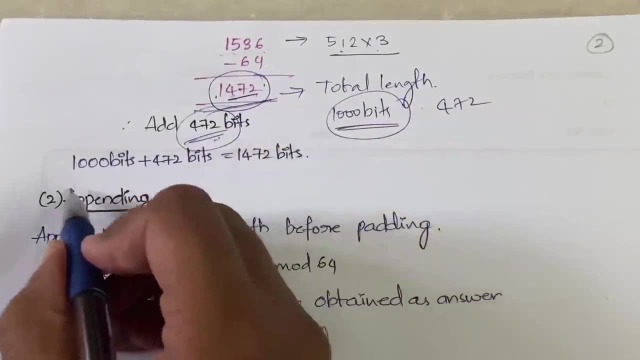 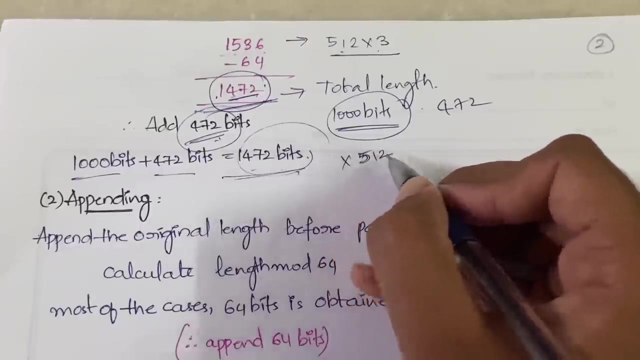 original message that you have that is of 1000 bits, right? so we already have 1000 bits. so additionally, how many bits? you have to add 472. so additionally, you have to add 472 more bits. so 1000 bits plus 472 total will give you 1472, which is multiple of 15. sorry, multiple of 5 and 2. 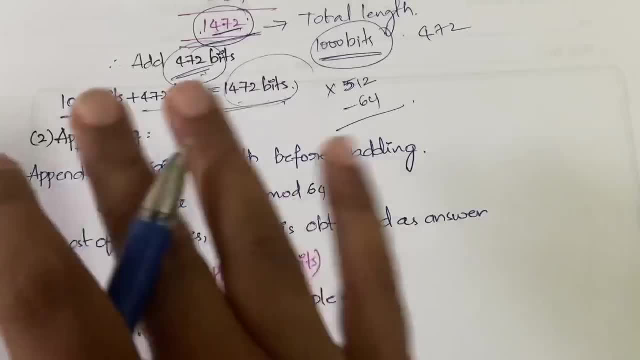 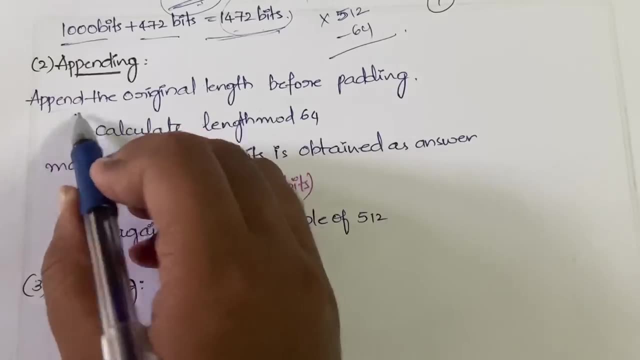 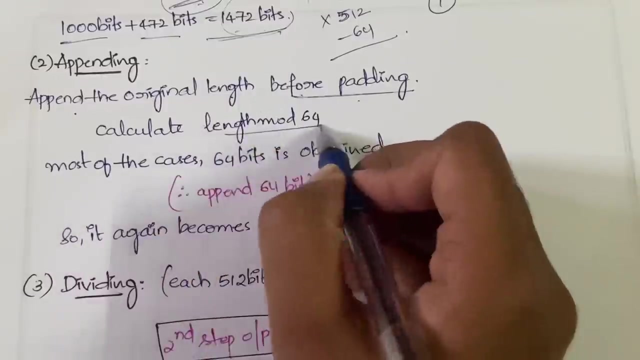 and also 64 less got it. now we are done with the first step, that is, padding. now second step is nothing but appending, appending, in appending. what you have to do is you need to append the original length before padding, okay. so what is the original length before padding? length mod 64? you have to do. 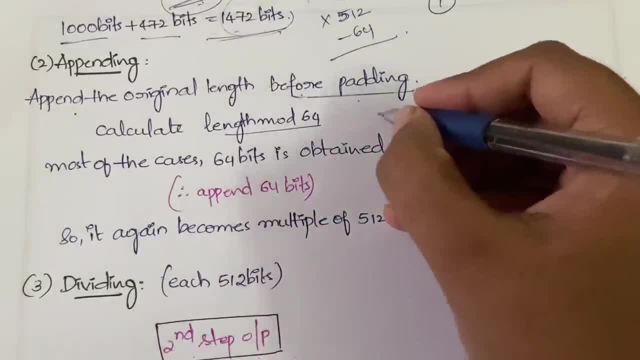 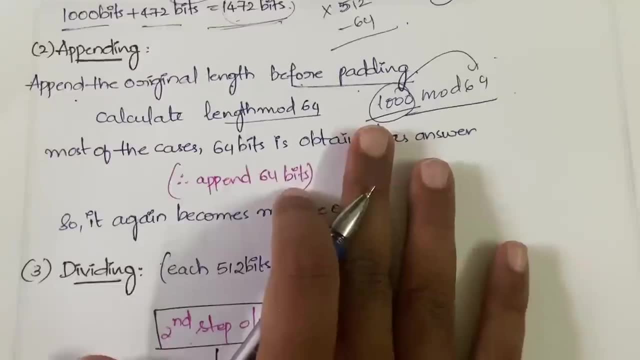 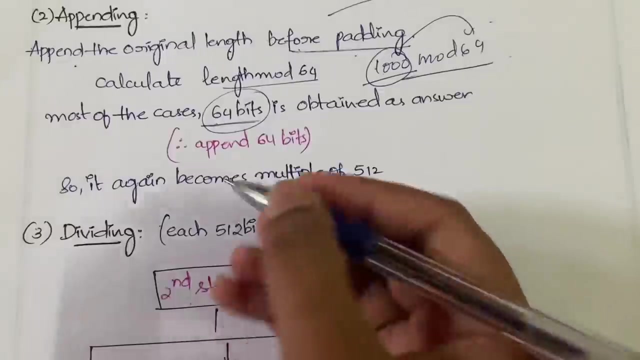 length is nothing but the original length, whatever it is. in our case it is 1000, right? so so 1000 mod 64. you should do so. whatever is the original length that mod 64 you have to do. in most of the cases you will be getting the answer as 64 bits only. okay, so that what you have to do then. 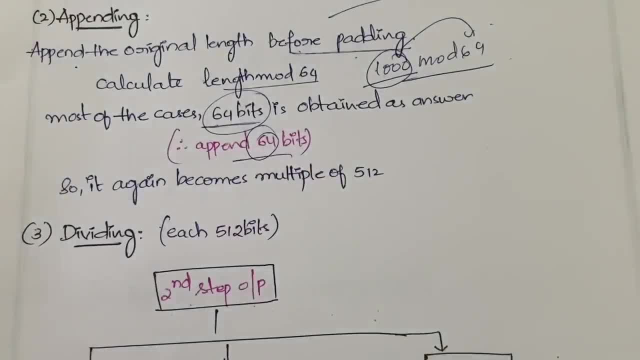 you need to append 64 bits again so that it will again become multiple of 5 and 2. that is, you are adding again 64 less in the previous step. what we have done, we have my subtracted 64. right now we are going to add 64 again back because in most of the cases you will be getting the answer as 64. 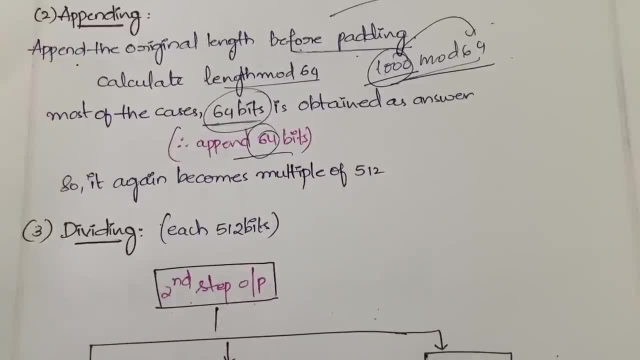 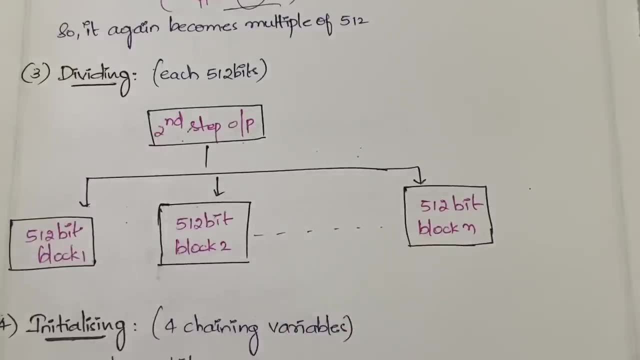 when you do this. so that is the original length that you have to do in the previous step. what we have tomorrow: you do this. okay, you got it. now. in the third step, what you have to do is you need to divide the entire message. you- whichever you have- you have to divide it into a number of sub blocks. okay, got. 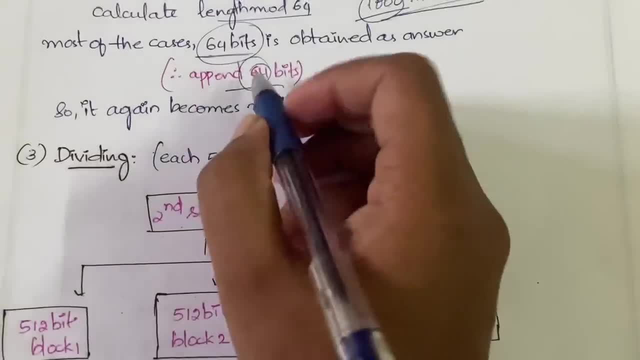 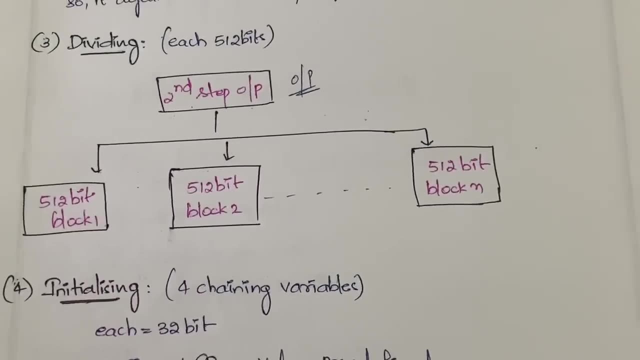 it. so, whatever the output that we are going to get in the second step, that is, after up pending, the 64 bits, whatever output we get back again. so for that, what you have to do is this: 64 bits to what you have to append to this: 147 creativity, which is 64. so, looking ahead, you will see we are stop by to this. second. you look at this 64 bits exactly. we are not going to head back down in the next slide, we are going look at this 64, we are going to forward it. just for short, the prom does not have the most important visual airflow. we want to know this and this is the top we have to increase. but you know, during this you only have to. 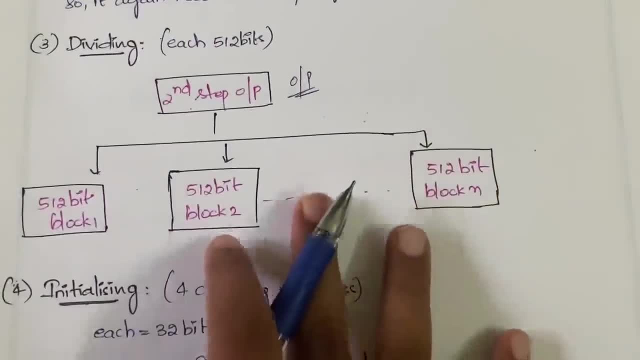 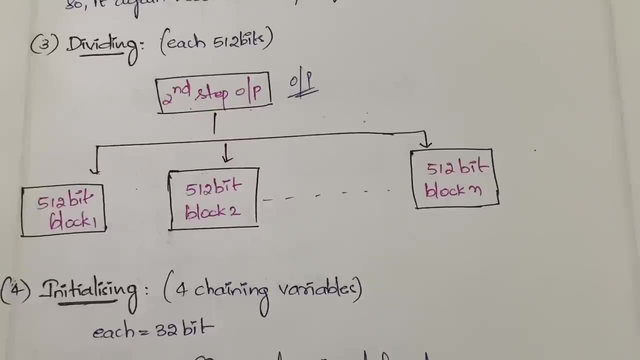 1472 again back right. so when you append that again to that, you will be getting again a number which is multiple of 512, because initially you have subtracted 64 and now you are adding 64, so done, you will be getting a multiple of 512 at the end. now what you have to do is you need 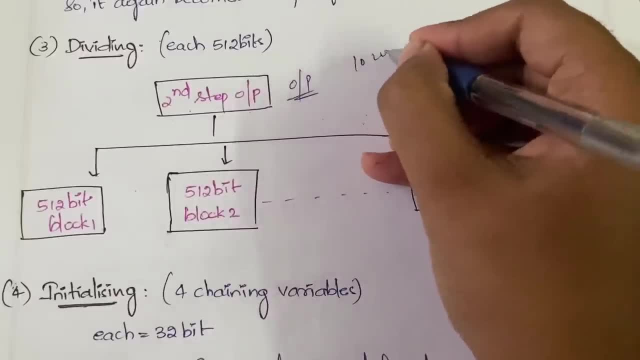 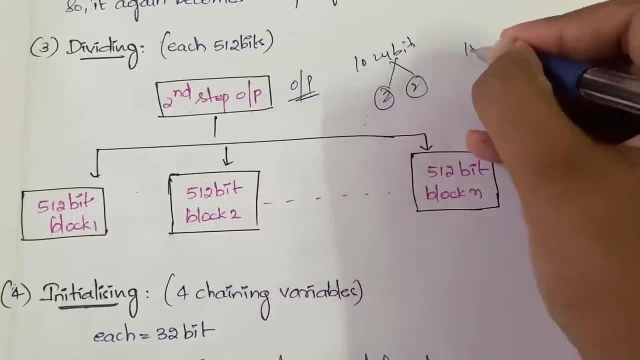 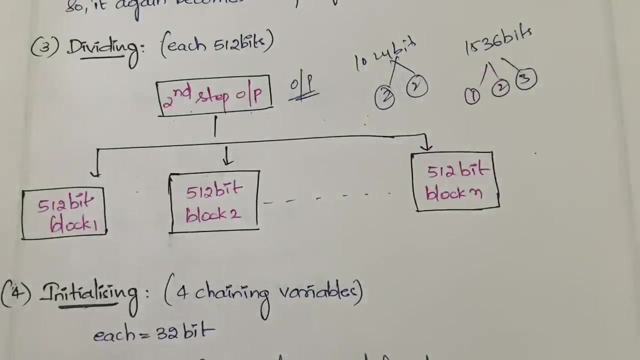 to divide it into number of sub blocks. if you are having only 1024 bits, in that case it can. you can divide 512 into how many parts. you can divide it into two parts. we are having 1536 bits. then in this case, what you can do, you can divide it into three 512 bit blocks. right, so that, based on the 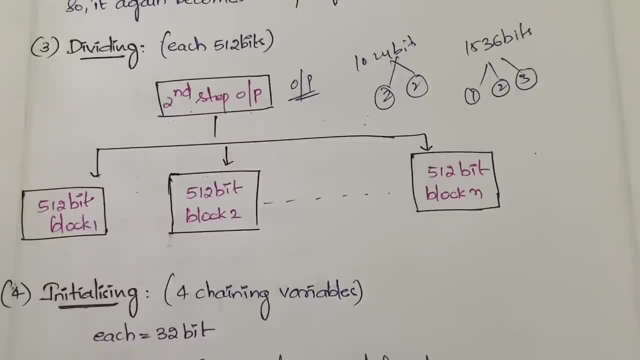 length of the output. you can divide it into sub blocks with each length 512 bits. got it now in the third step. we have done the division dividing as well. now in the fourth step, what you do is in the fourth step you will be initializing the variables. you'll be taking four chaining variables. 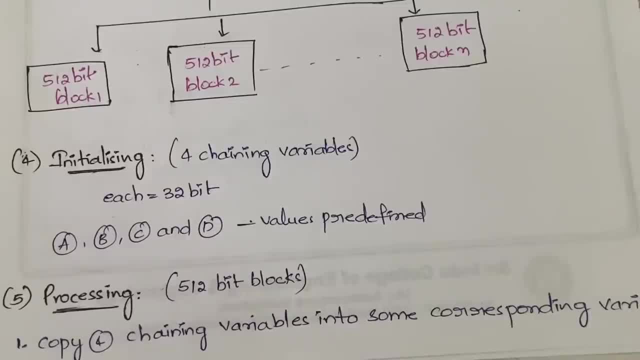 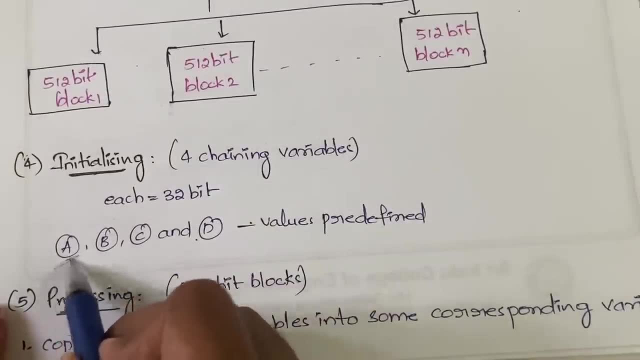 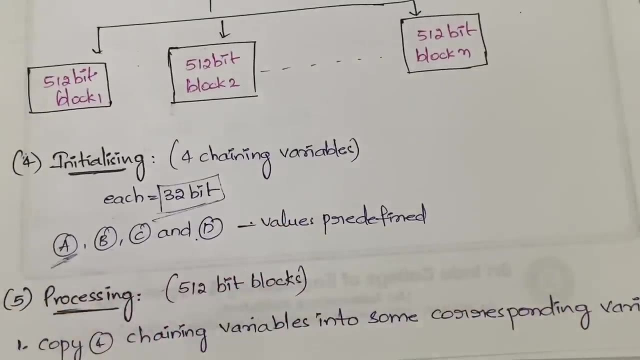 you will initialize those four chaining variables. got it, and you are representing those four chaining variables as a, b, c and d, and the length of each and every- yeah, the length of each and every variable is 32 bits. got it now, and these chaining variables will have the predefined values itself. previously, only we have a predefined values. 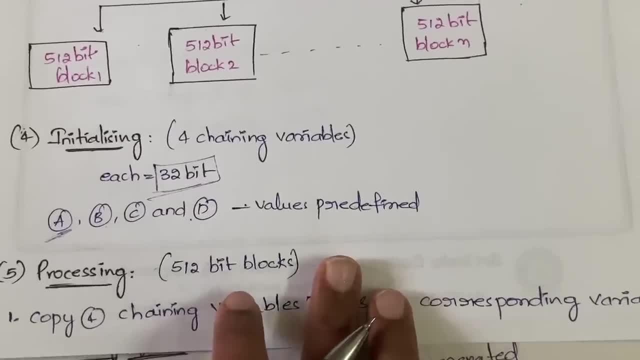 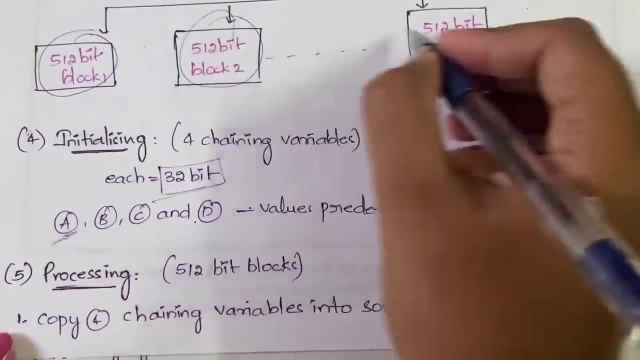 for them, got it. next. what you have to do is you need to process these, processing in the sense what you have to process, not these chaining variables. this blocks this 5 and 2 bit blocks, what you have divided. you need to process them now. processing in the sense in the first step. 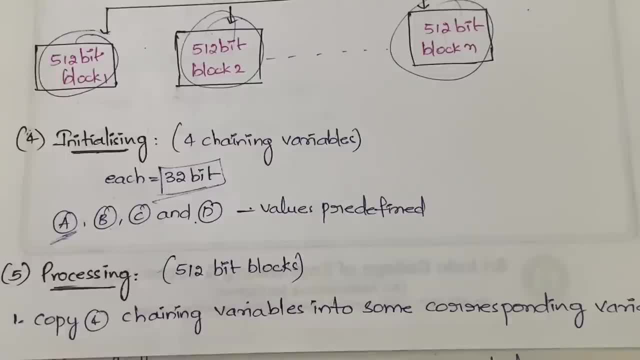 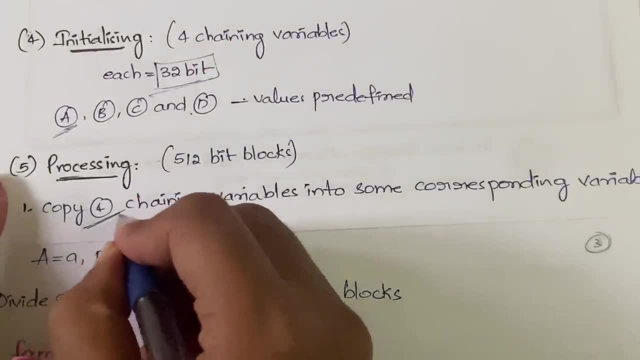 what you have to do is- and again in the processing also, we have several steps. first, what you have to do is you need to copy those four chaining variables into some corresponding. first what you have to do: you need to copy these four chaining variables into some corresponding. 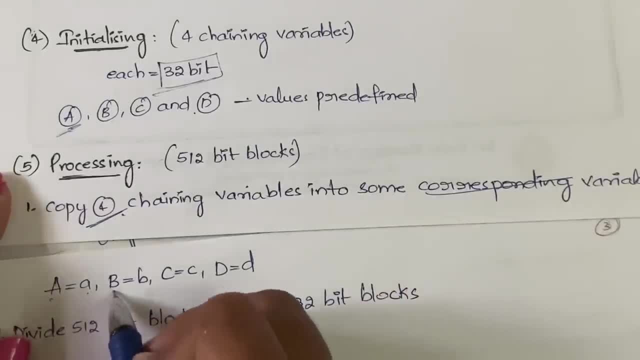 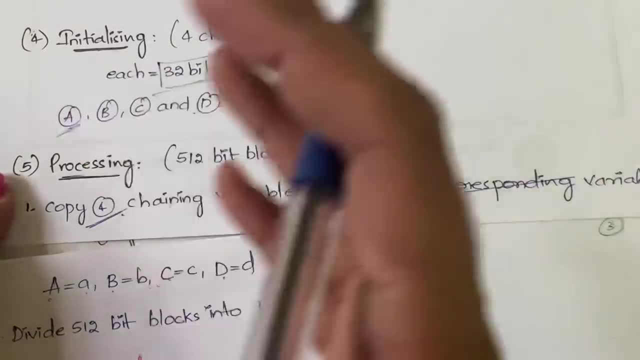 variables. see, we have done here: a is equal to a and capital b- cap small b. capital c- small c, capital d- small d, like that. we have copied them into some some separate other variables. got it now in the second step. what you have to do is you need to divide this 5 and 2 bit blocks into. 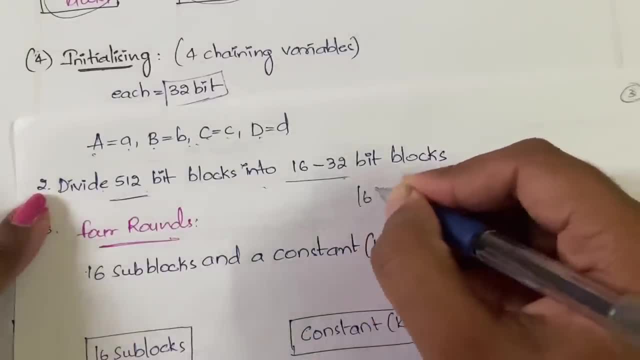 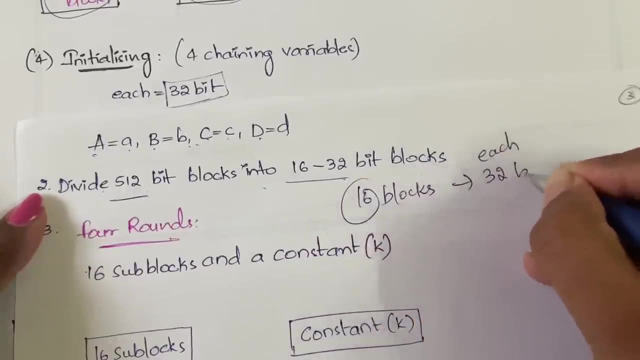 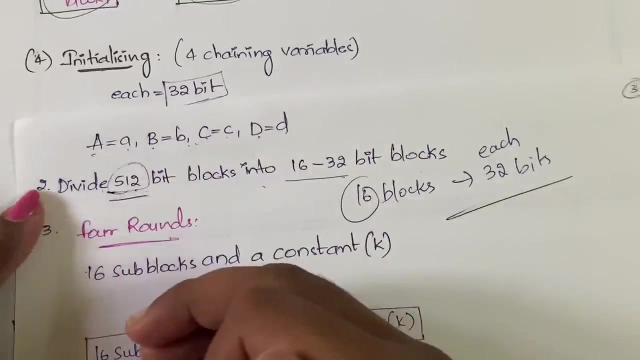 16, 16, the 32-bit blocks, that is, 16 blocks each of size. each of size, 32 bits got it. so, whatever the 5 and 2 bit blocks you're having, you need to divide them how. you have to divide them into 16 sub blocks and 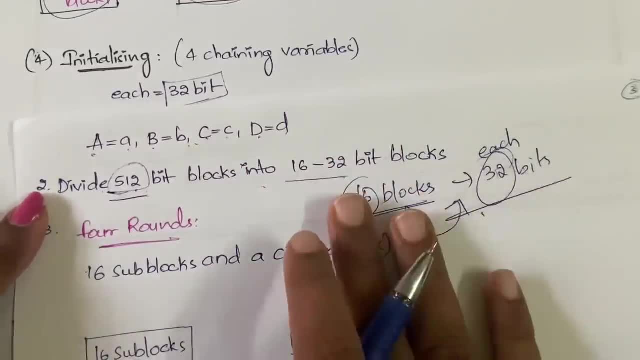 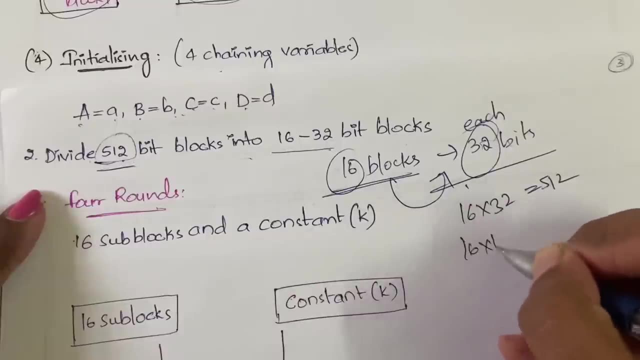 the size of each and every sub block should be equal to 32, got it. you just check 16 into 32 whether you will get 5 and 2 or not. you check see 16 into 16 into 2. we can write it as red 256 into 2. yeah. 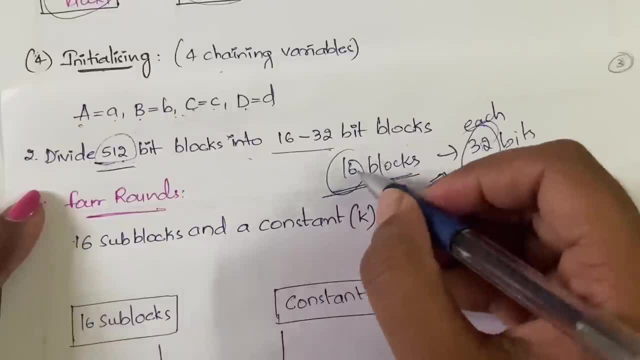 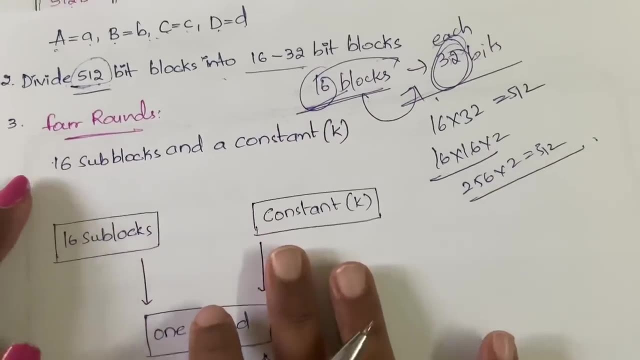 5 and 2 got it, so you need to divide it into 16 blocks, and each block having 32 bits as its size. none now in the third step, what you have to do is you'll have the four rounds here. so before telling photon what is that? 4 rounds and all? i'll just uh tell you in simple way. so here you are, having a 16. 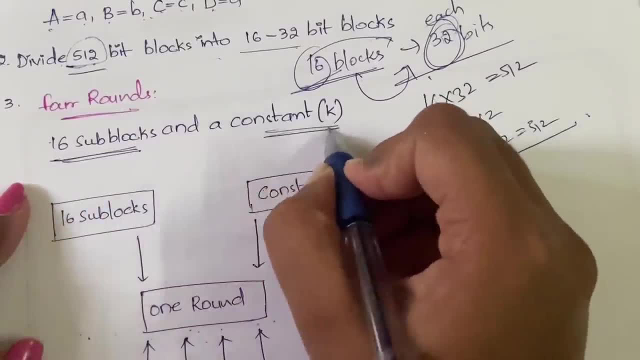 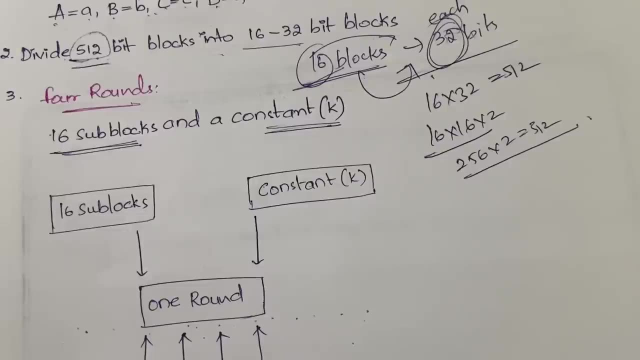 sub blocks. right, and you will also take a constant, okay, okay, constant, which is represented with the help of k or p, whatever constant as you can have them alternatively. so now let's see how we have this. whatever constant, according to your convenience, you can take any constant, got it? so what do you? 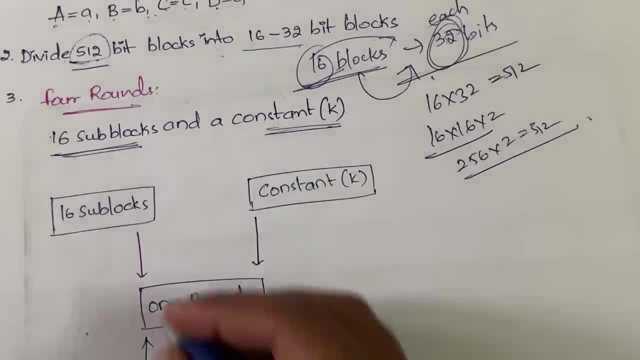 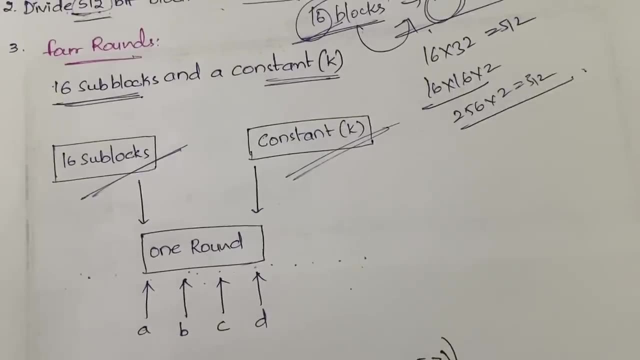 have here? what do you, what do you have as the input? here you have the 16 sub blocks and also you have a constant. so in each and every round, what happens is you will also give this four chaining variables, also as input got it. so, when you give this four chaining variables in each and 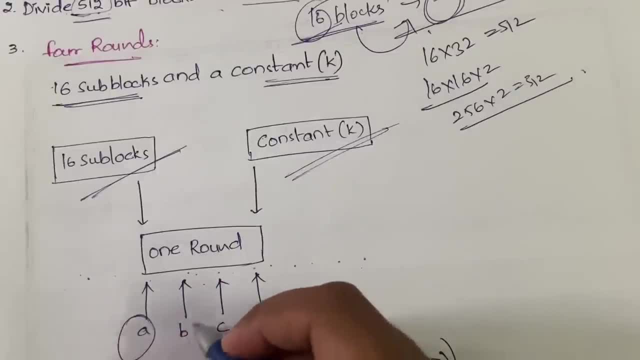 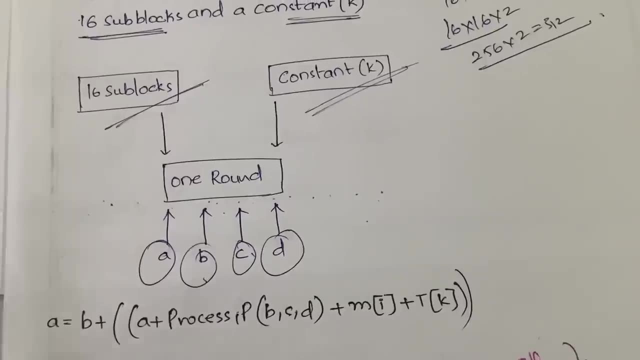 every round one, one variable will be calculated. in round one you calculate a, and round two you calculate b. in round three, you calculate c and in round four you calculate d. and how do you calculate that? i'll tell you see, a is equal to b plus b plus a into process which is denoted by p. 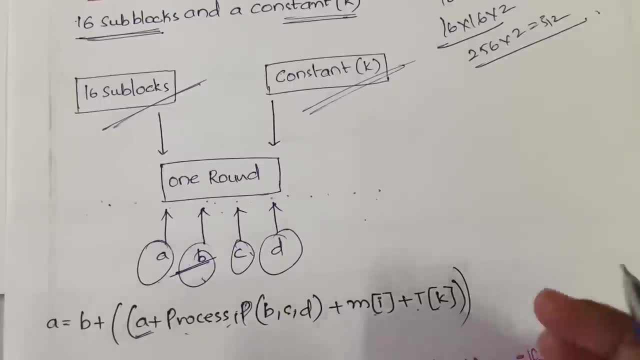 of bcd plus m of i plus t of k got it right. so this is the, this is the process, this is the way how you calculate a. in the second round you will be doing it for b. so here a will be replaced by b. here you get a, and here you get b again, and here you get a again. so like that, so in each and every. 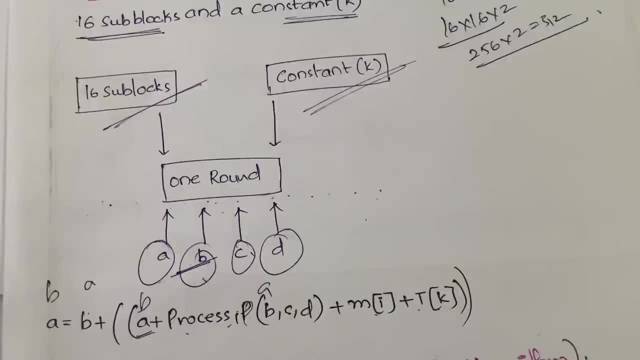 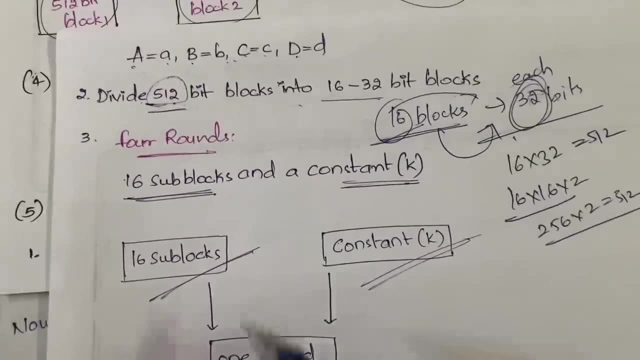 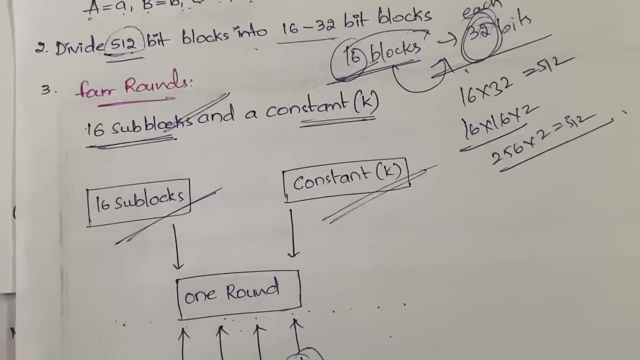 round, you will be calculating the each and every chaining variable. got it: a, b, c, d, so we have four variables. that is why we have to perform total of four rounds, got it. so this is all about this video. this is all about this message. digest five algorithm. got it. you are dividing your message. 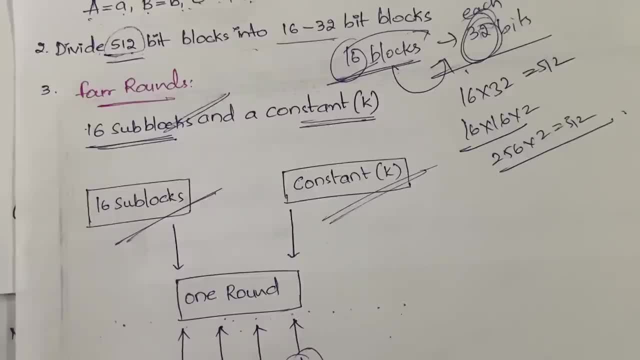 into number of sub blocks, number of digest you are breaking down, right. that is what the ultimate theme of message digest is. got it. now, after this message digest, we are going to learn sha algorithm, which is very short because it is completely based on this algorithm. got it? so that's all for this video and thanks for watching the video.